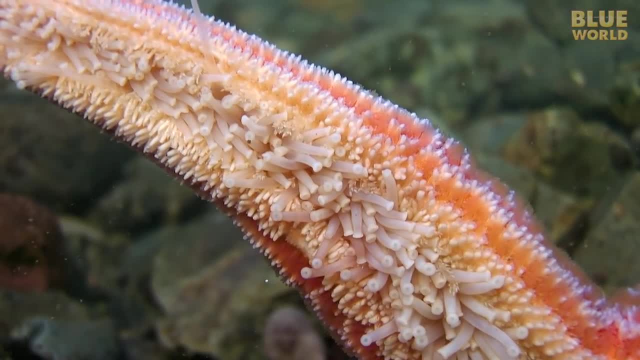 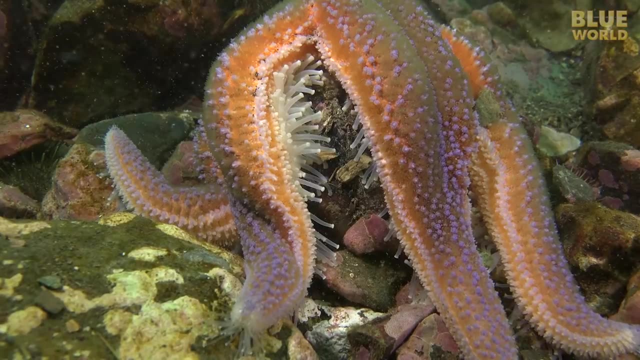 The animal has muscles in the tube, for example, and the water vascular system is used to retract the tube feet. By expanding and retracting the right tube feet in the proper order, the animal can walk. Many echinoderms can also form suckers on the ends of their tube feet used to 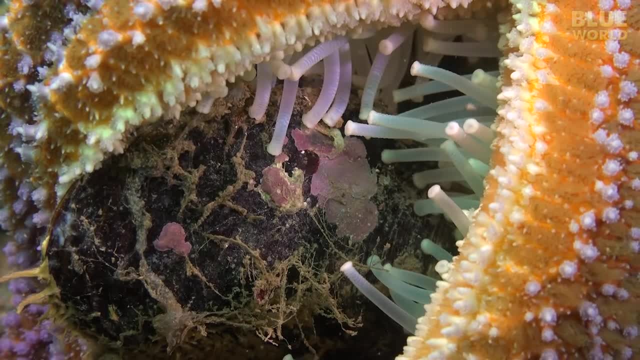 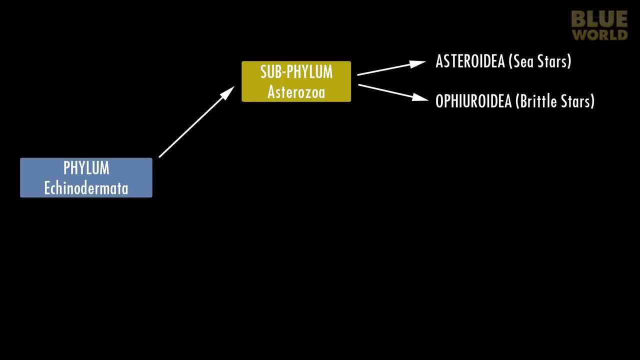 capture and hold prey or to hold onto rocks in a swift current. The phylum is broken up into three groups: the subphylum Astrazoa, the class Crinoidea and the subphylum Echinazoa. the Asterozoa are, as you might imagine, the star-shaped animals, Since they aren't 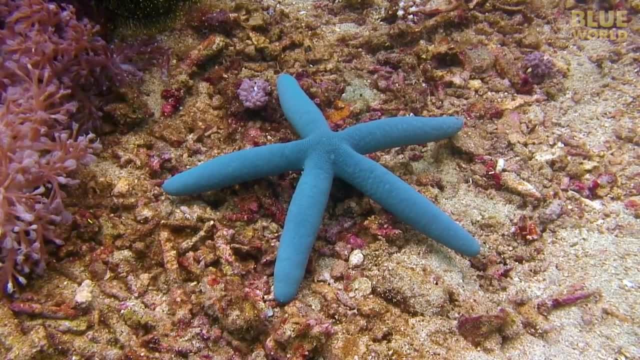 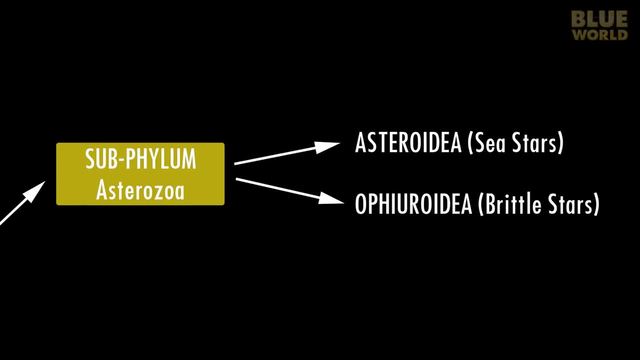 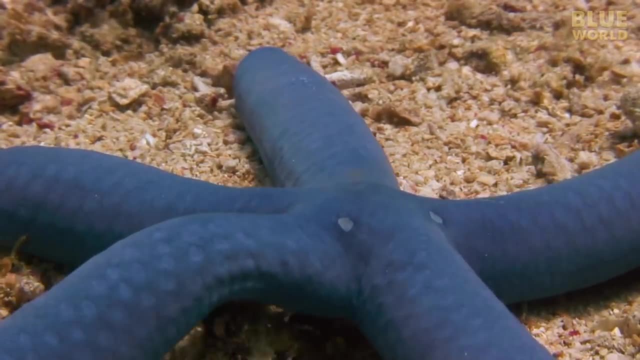 actually fish. the correct term for these animals is sea stars, not starfish. Within this group there are two classes: the Asteroids and the Ophuroids. The Asteroids are the sea stars that have thick arms and no recognizable central body. The Ophuroids have thin arms. 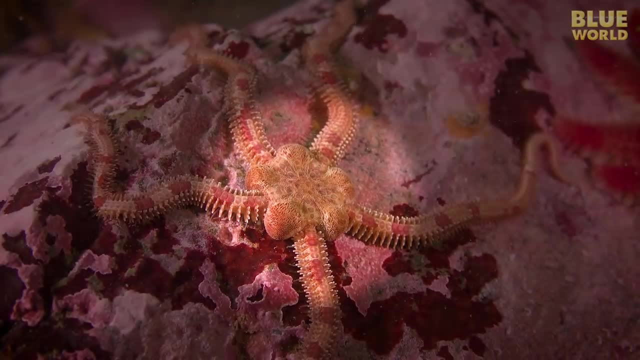 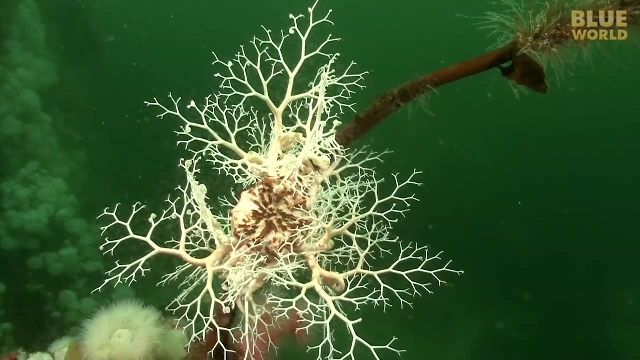 and a distinguishable shape. They have long, thin arms and will be shaped similar to the central body part. Offuroids include the brittle stars and basket stars. Brittle stars and basket stars generally use their fine arms to catch plankton from. the water rather than hunt larger prey, like asteroids generally do. Most tropical basket stars are nocturnal. They only come out at night, when the plankton is most abundant. They're sensitive to light and hide the minute I light them up with my camera. 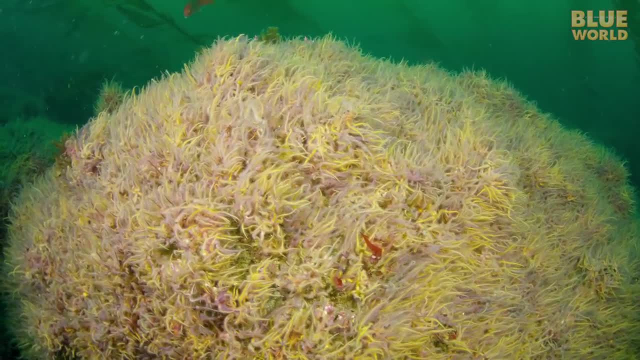 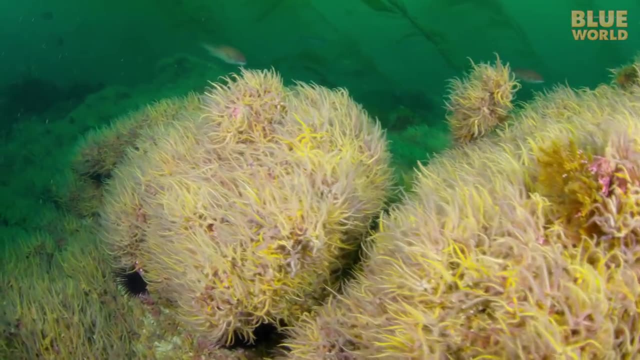 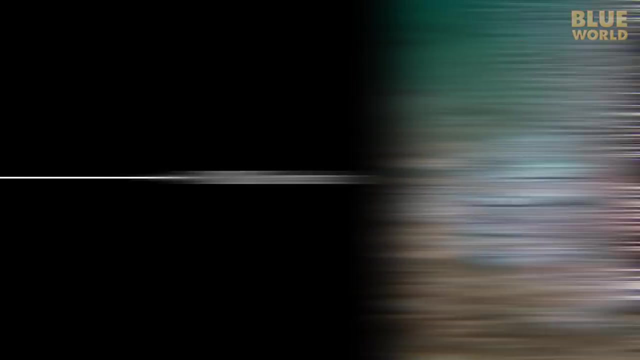 In California, immense beds of brittle stars stick their arms into the current for food. This is a landscape dominated by brittle stars. The crinoids, known as feather stars, are distant relatives of the sea stars, Like the offuroids. their arms are feathery, which makes them even better than brittle stars. Feather starshat catching plankton like a living net. Feather stars are quite common in the tropics, where they tend to find a good place to perch and catch plankton. The food is moved to the central mouth by cilia. They are also. 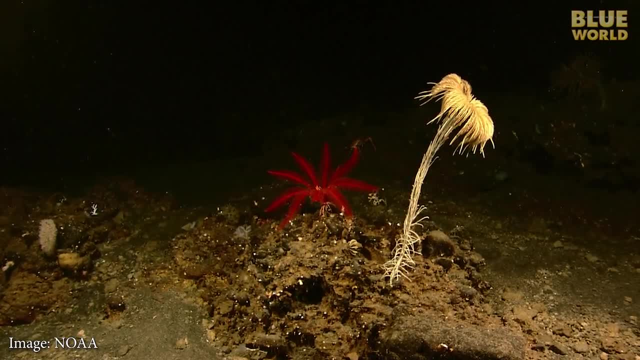 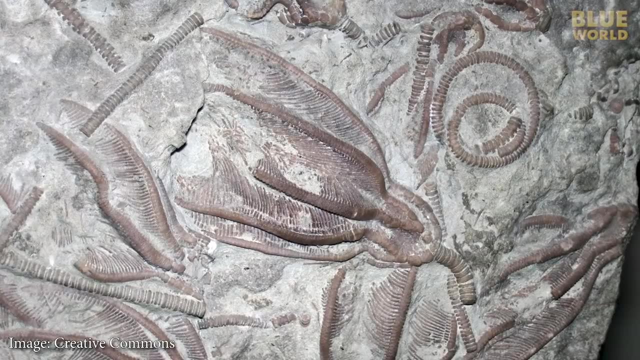 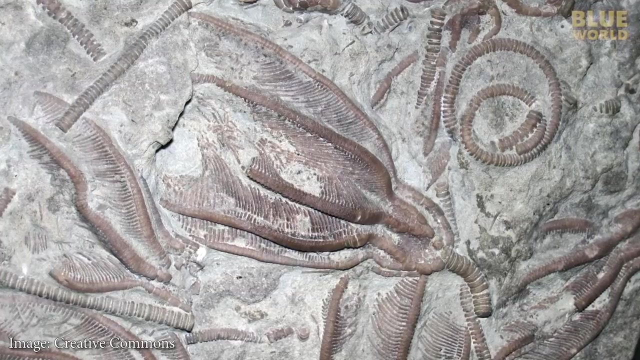 well represented in the deep sea, where they tend to have stalks to allow them to get higher up off a flat seafloor. They go back almost 500 million years in the fossil altered, so crinoids have been around a long time. 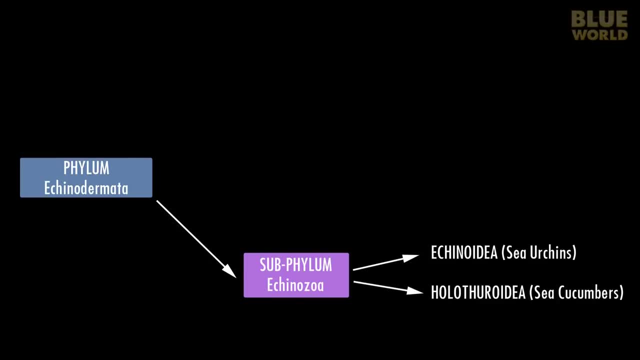 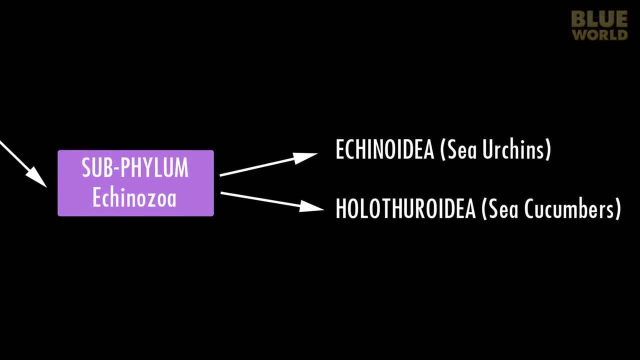 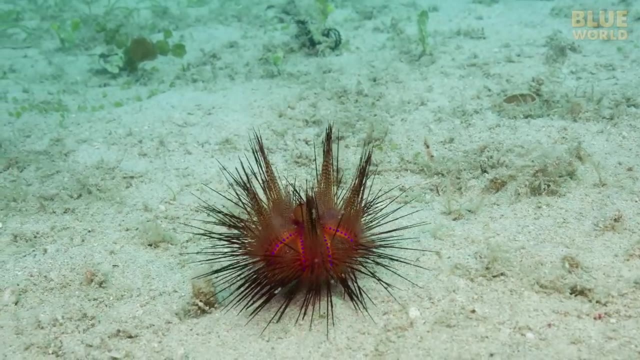 The last subphylum is the echinazoa. This group includes two classes: the echinoids and the holotheroids. They are related through common evolution, but they are very different. The echinoids, which have the spiniest skin of all, the echinoderms includes the sea urchins. 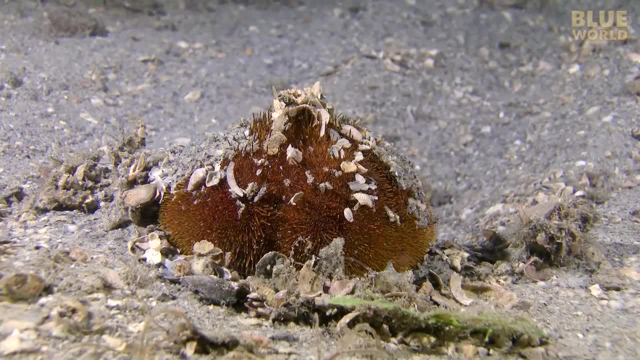 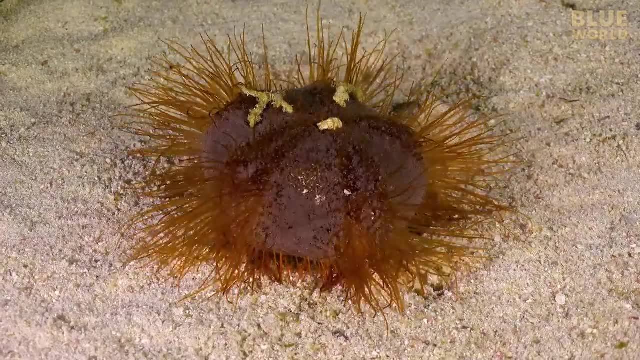 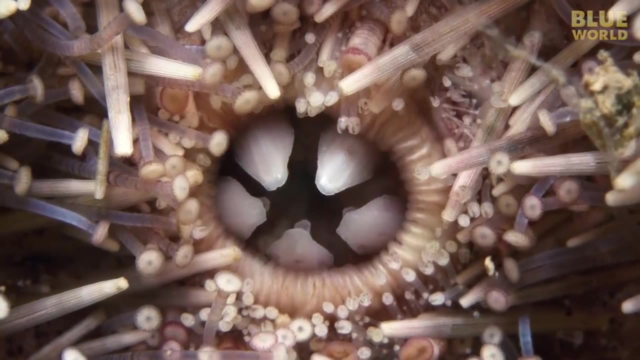 and their relatives, the heart urchins and even the sand dollars, which are basically flattened sea urchins with super short spines. Sea urchins also use their tube feet for locomotion. like sea stars, They have a mouth on the underside with teeth for chomping on algae. And when the food supply is good, the urchins multiply. Having all those sharp spines makes a good defense, not only for the urchin itself but for animals that can fit between the spines. Urchins often have fish, shrimp and other small animals. 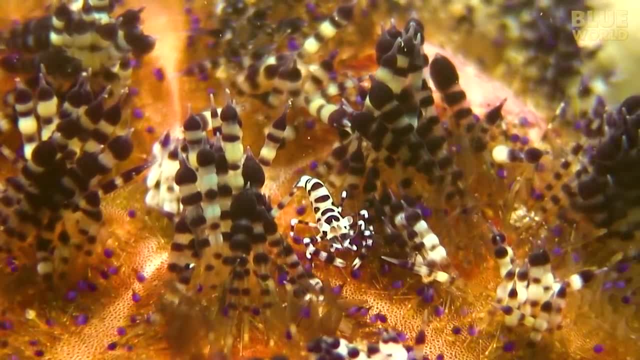 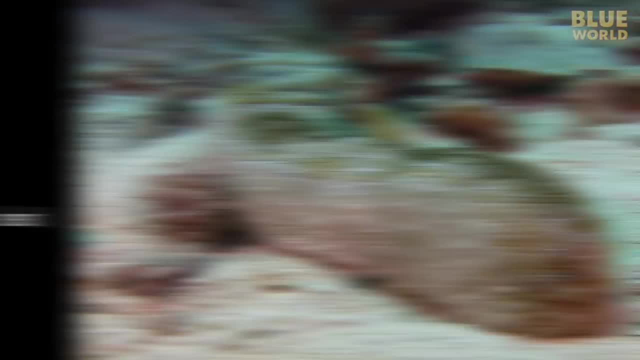 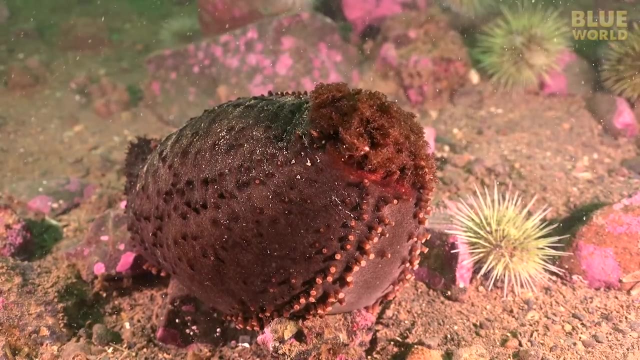 The class holotheroidea is composed of creatures called sea cucumbers. A sea cucumber is so named due to the fact that many members of this group resemble the garden variety of cucumber. They also don't really have spiny skin, so they are the exception to the echinoderm's. 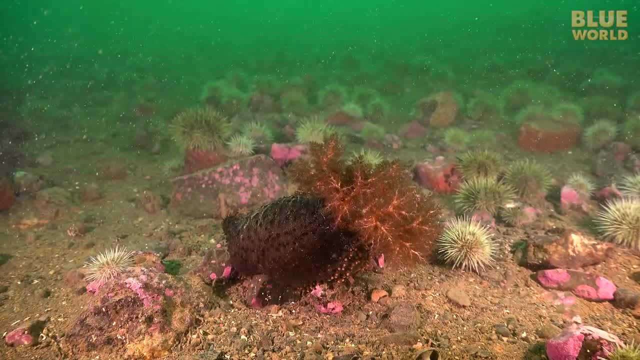 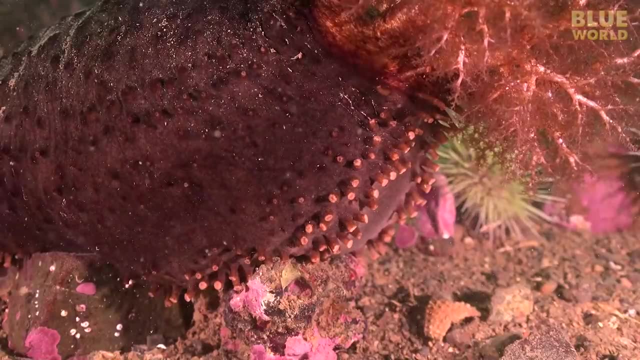 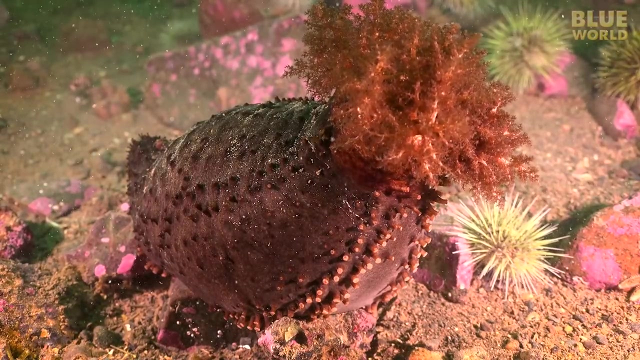 spiny skin rule. But other anatomical features make it obvious that sea cucumbers are clearly related to the other echinoderms. For example, they have tube feet. Sea cucumbers are often somewhat football-shaped and lay on their side on the bottom. 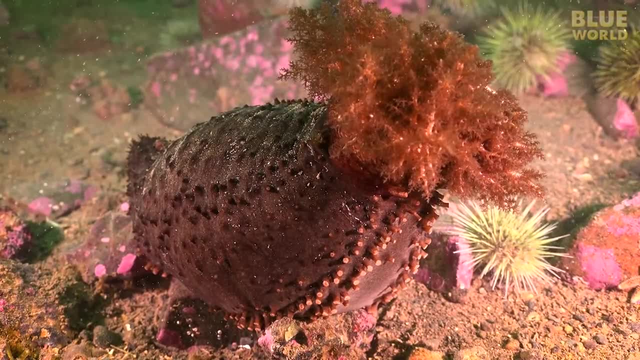 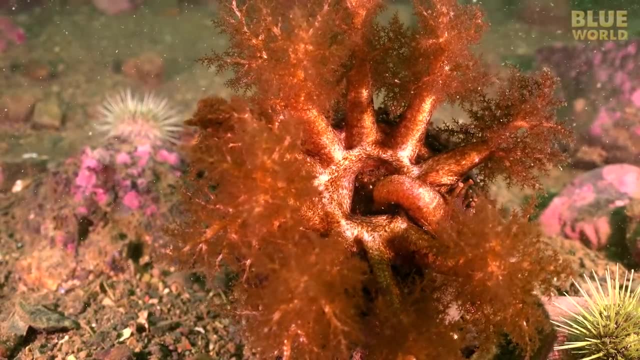 They have five rows of tube feet running lengthwise like the seams on that football. At one end of the animal is a mouth surrounded by tentacles. These tentacles are also tube feet, specially developed tube feet used for feeding. These tentacles are also tube feet, specially developed tube feet used for feeding. 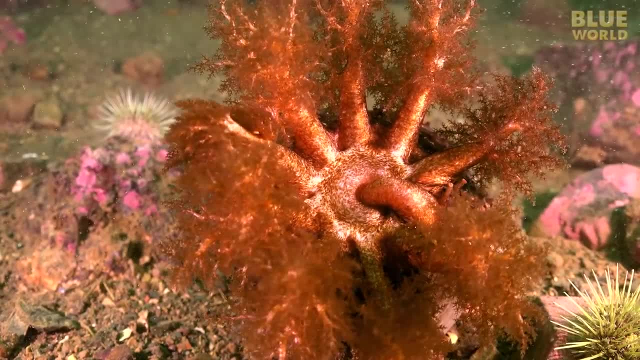 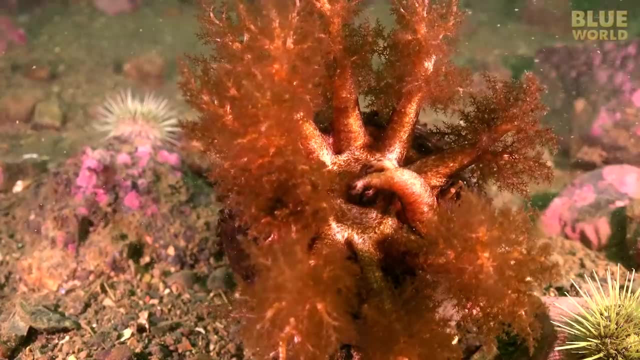 These tentacles are also tube feet, specially developed tube feet used for feeding. Some sea cucumbers use them to feed on plankton. The tentacles collect food from passing water. Then the cucumber sticks each tentacle in its mouth, one at a time, and licks them off. 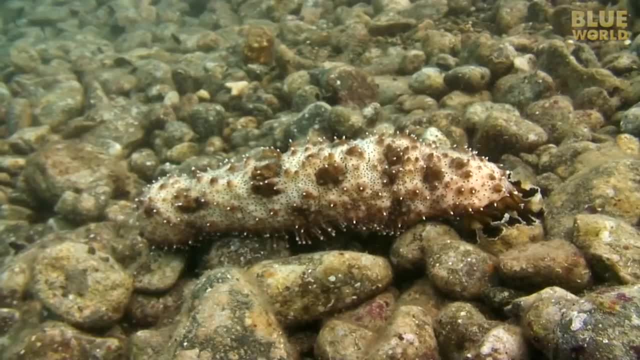 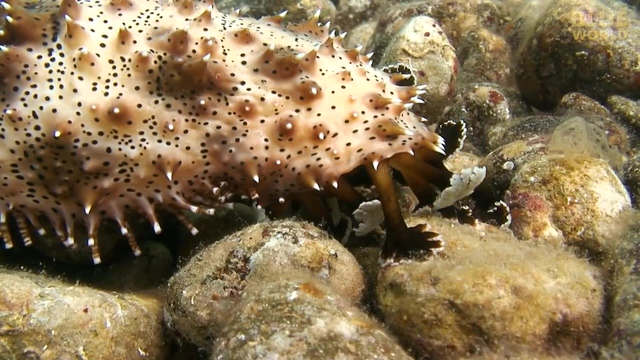 Mmm, yummy plankton. Other kinds of sea cucumbers use the tentacles to sift through sand on the bottom for particles of food. You might think that an animal like this would be defenseless. It has no spines like a sea urchin. 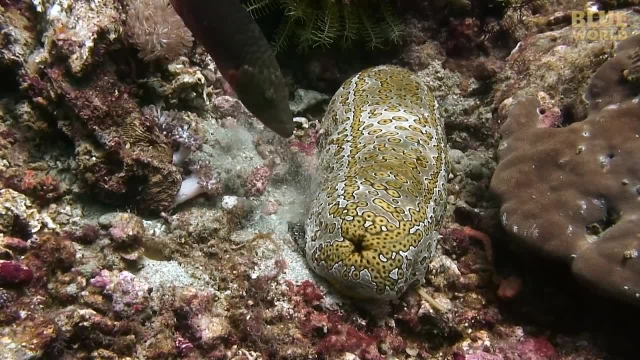 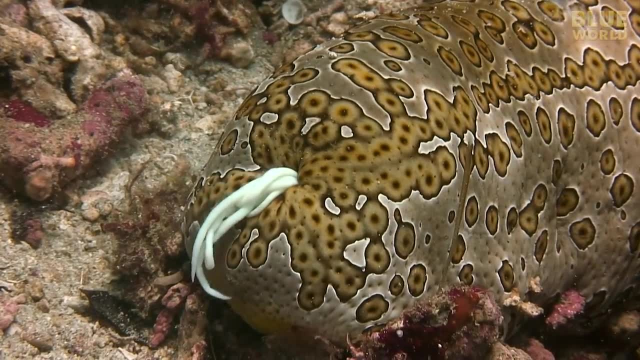 It doesn't even have tough, spiny skin, It just looks like a soft, squishy, bite-sized meal. But when threatened, some sea cucumbers can eject a sticky, disgusting goop called cuvarian tubules to ensnare predators.